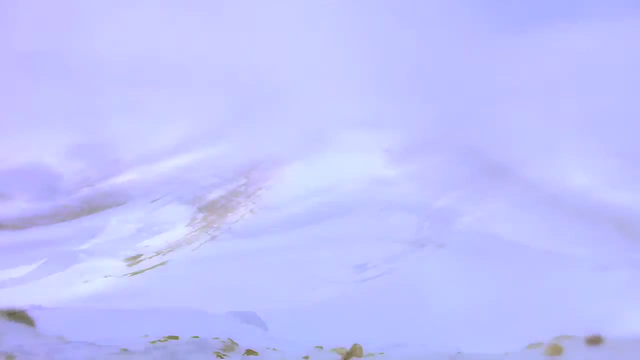 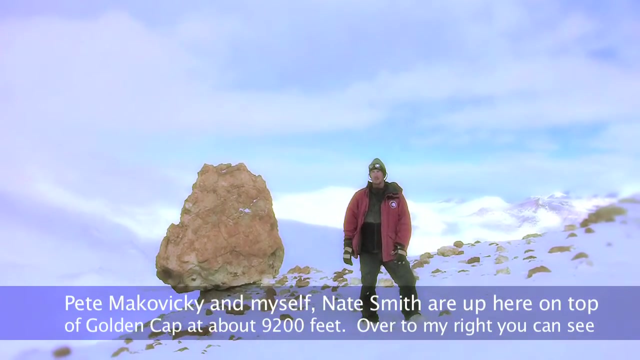 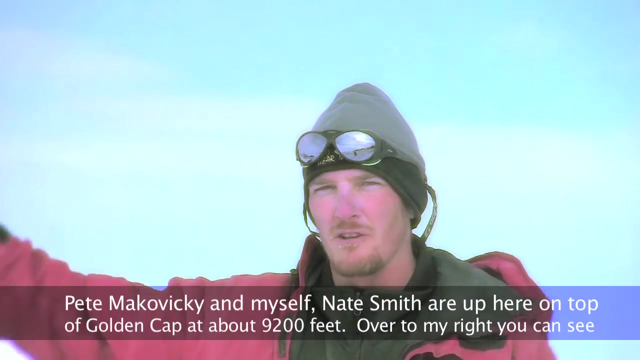 Henson Formation Sediments. Hey, so me, Mack and Vicki, and myself, Nate Smith, are up here on top of Golden Cap at about 9,200 feet Over to my right. you can see Hansen Spur and Mount Vala that are clouded. 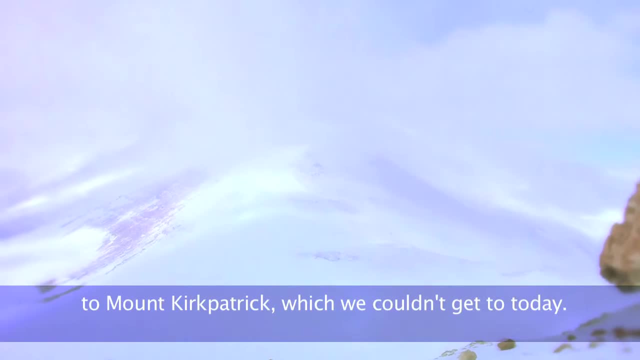 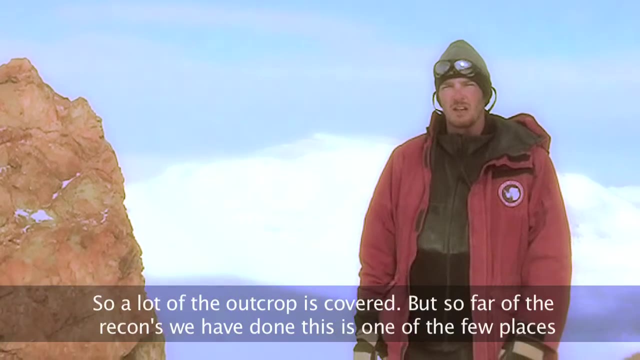 in. You can see those clouds extend all the way over to Mount Kirkpatrick, which we couldn't get to today. Golden Cap: not much is exposed right now Because we've gotten a lot of snow in the past week, so a lot of the outcrop is actually. 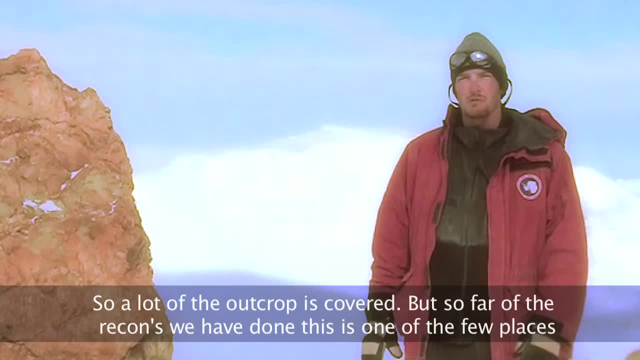 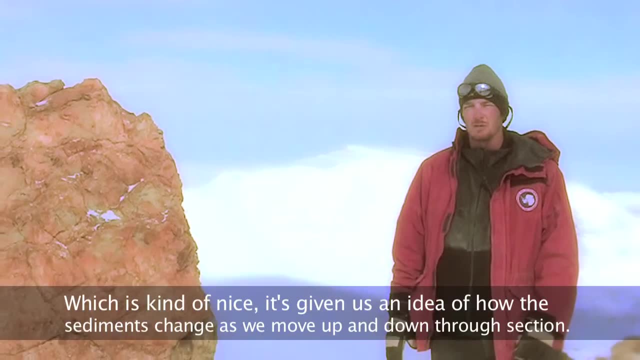 covered, But so far of the recons we've done, this is one of the few places that we've been able to walk through the Hansen Formation and down into the Vala Formation continuously, which is kind of nice. It's given us an idea of how the sediments change as we move up. 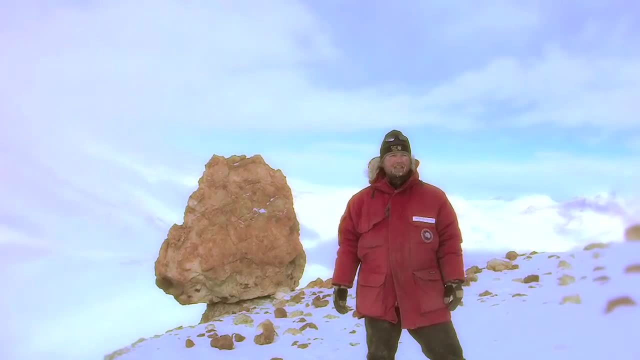 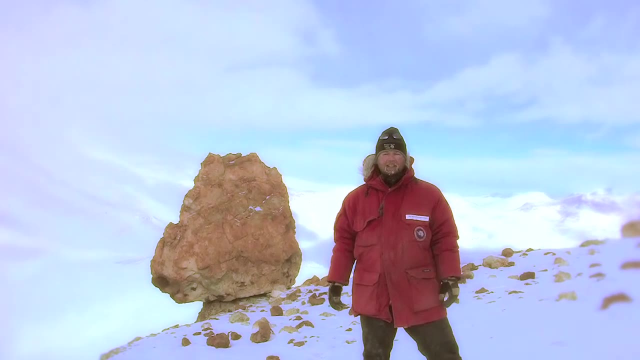 and down through sections. Nate and I have had a fairly good day up here on the mountain. Fortunately we didn't find any bones, but we did find some interesting beds. It might actually tell us a little bit about time and environment, So we collected a few. 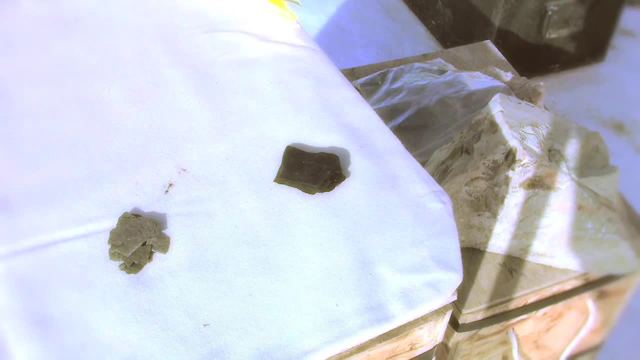 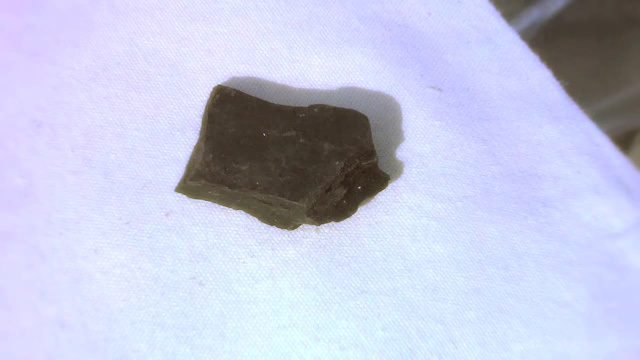 hand samples. there We collected rock samples from the Hansen Formation and the Vala Formation below it. These samples are rich in organic material, giving them a dark, almost black color. Eva Koppelhus, who is our team palynologist, will study these samples for clues about ancient 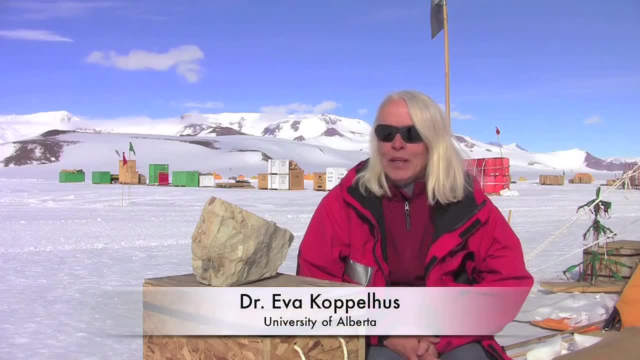 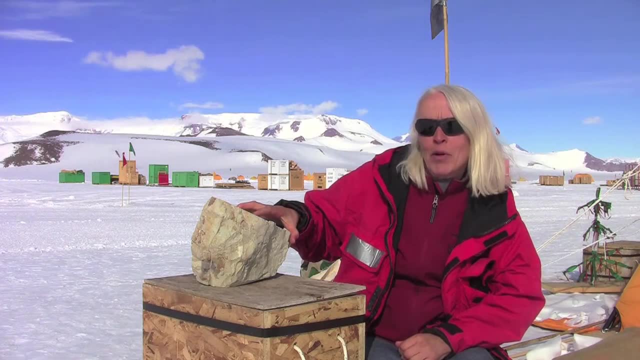 environments and also the age of the rocks. I'm Eva Koppelhus and I come from Canada. I'm a palynologist. The reason why I came along here is that I'm going to see if I can find any spores and 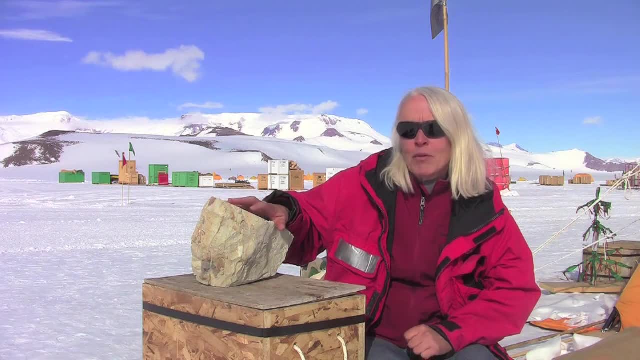 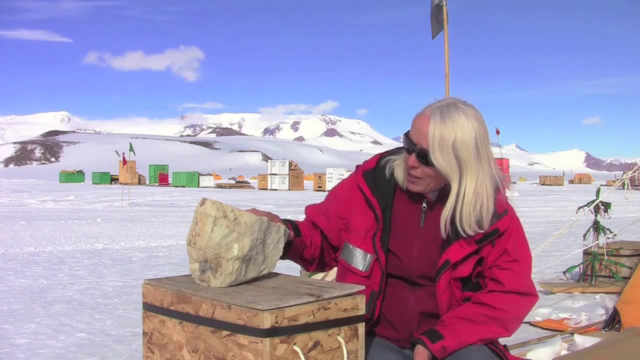 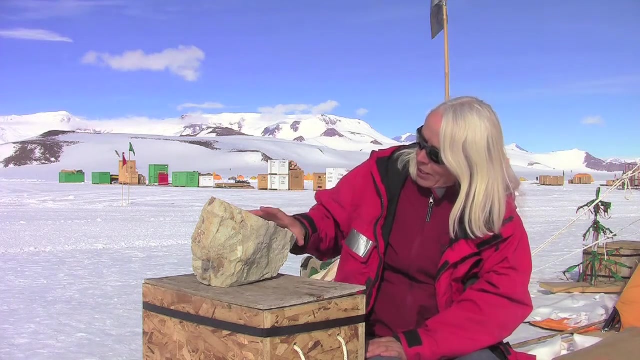 pollen in the Hansen Formation in the quarry where the cryolophosaurus has been found. So this is a piece from the quarry and, as you probably can see, it's first of all very hard rock and then it has a very light color and that's a bad thing for palynology. 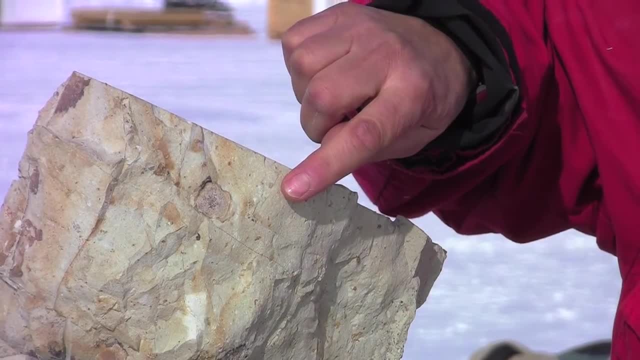 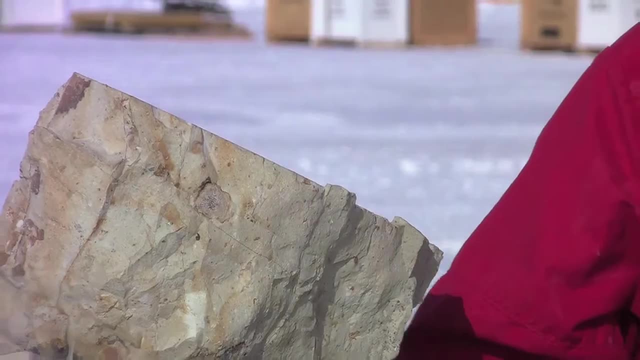 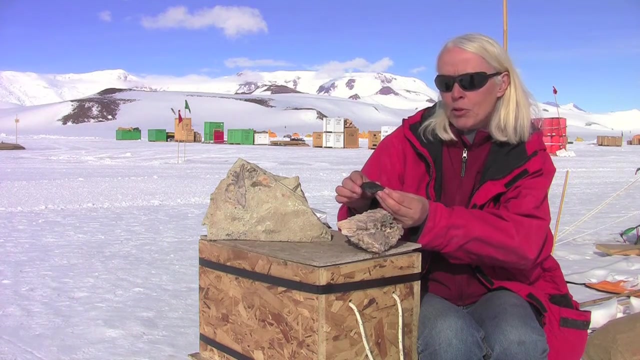 If you look closely here, there is absolutely no indication of hard rock. There are no signs of dark stains or anything, and that is probably a sign that there are no organic material in this rock. I have an example here of a shale which is full of organic material, full of coal, small. 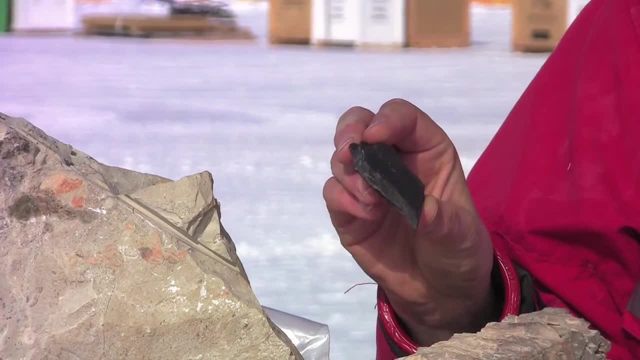 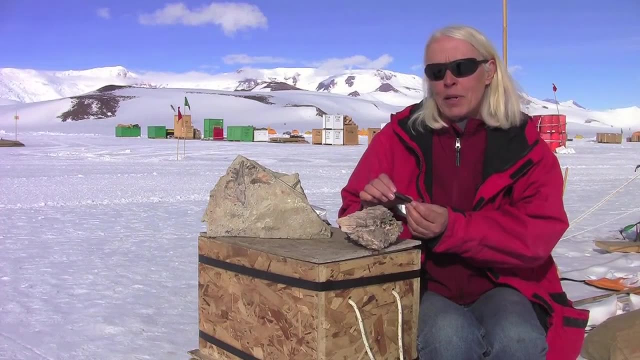 coal pieces and that is probably going to be really good for finding spores and pollen. The reason why I want to find the spores and pollen is so I can say something about what kind of plants that grew at the same time. The animals, the dinosaurs, were around. 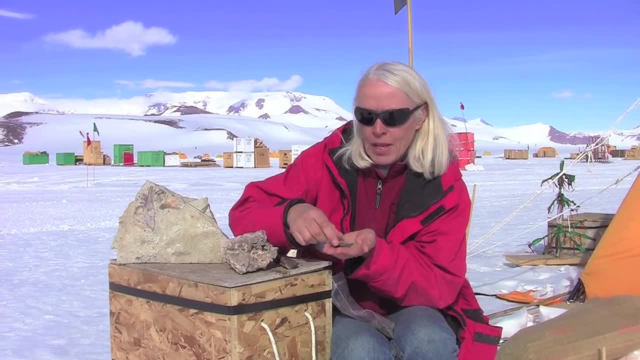 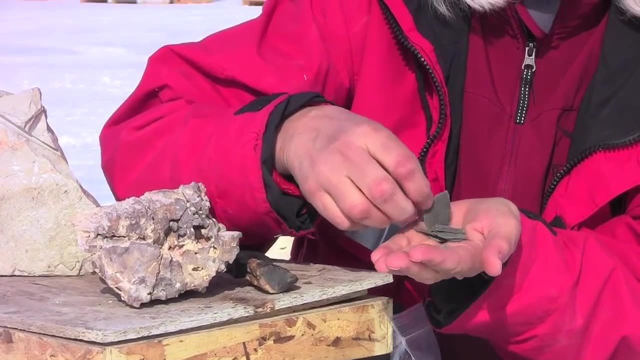 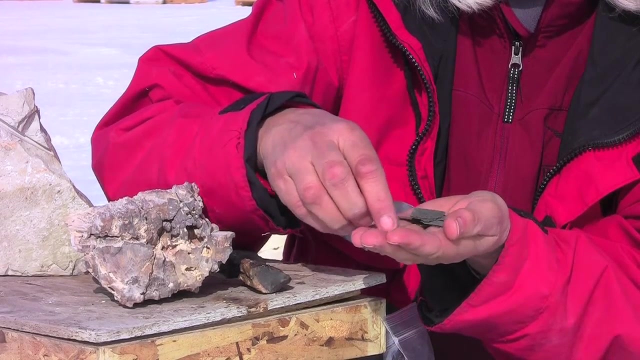 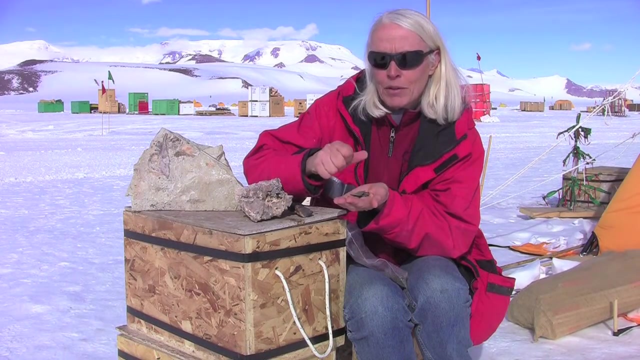 The process for analyzing these sediments for organic material is that you take sort of a small amount of it to the lab and then you dissolve all the minerals away with hydrofluoric acid and then you rinse what's left and that is the organic material and you in 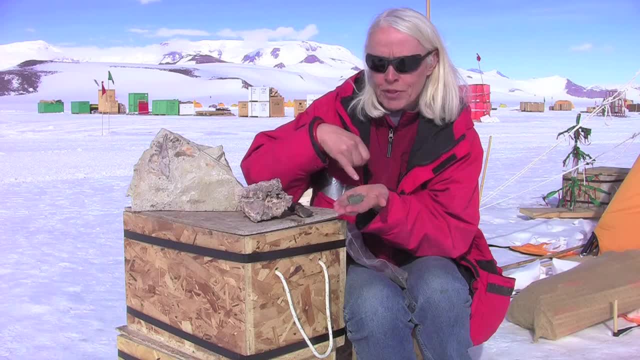 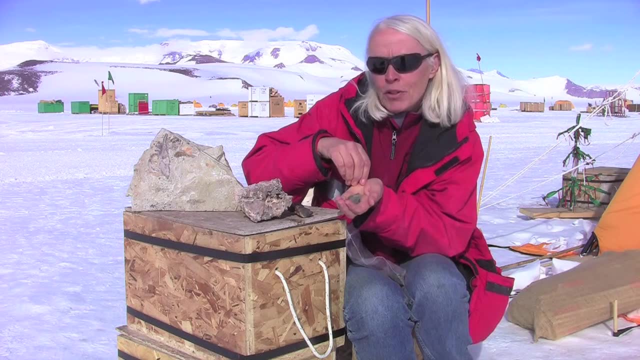 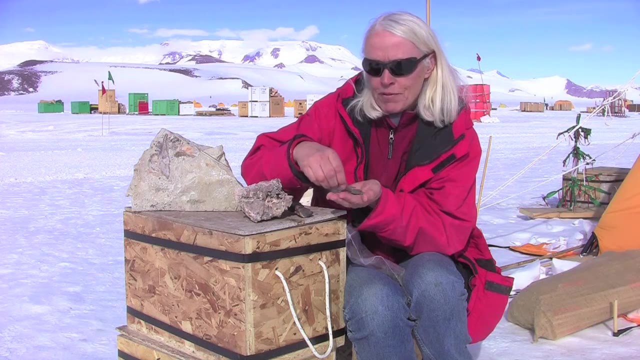 some cases you will color it to be able to see morphological features, but in other cases you just put it on a slide and then you study it under a microscope and in that way you can see what has been left of organic material there, and sometimes you can be very 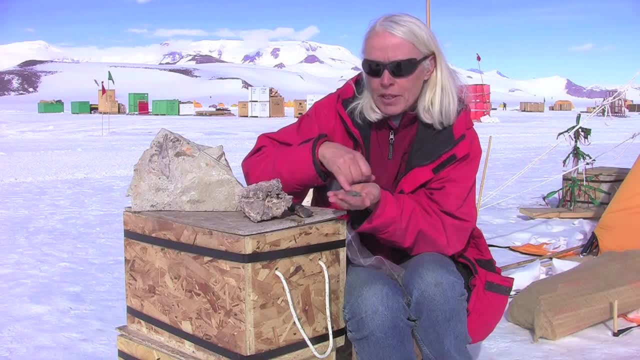 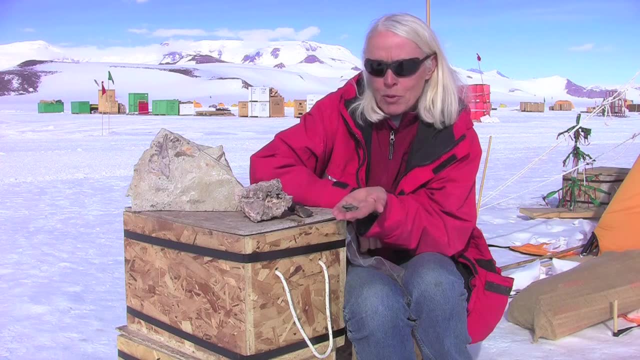 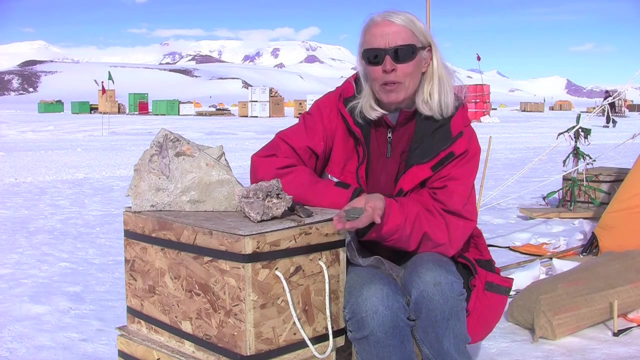 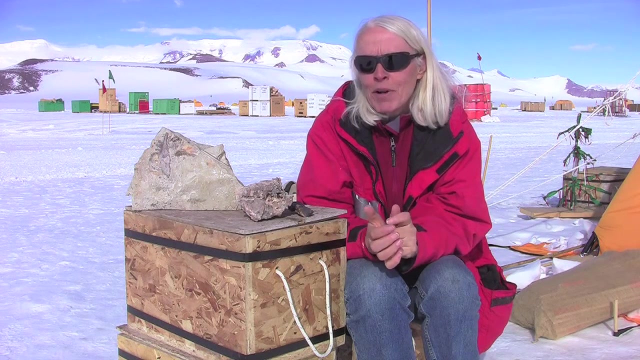 lucky and have very rich samples, and I am predicting that this is probably going to be a rich sample with lots of spores and pollen. It's a time-consuming job, but it's very rewarding when the samples are good. By finding out what plants there are, I can say something about the environment and I 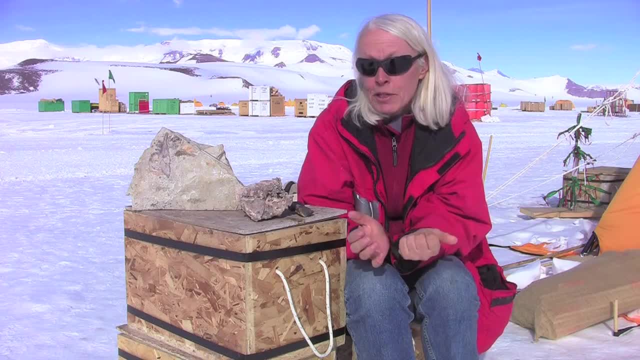 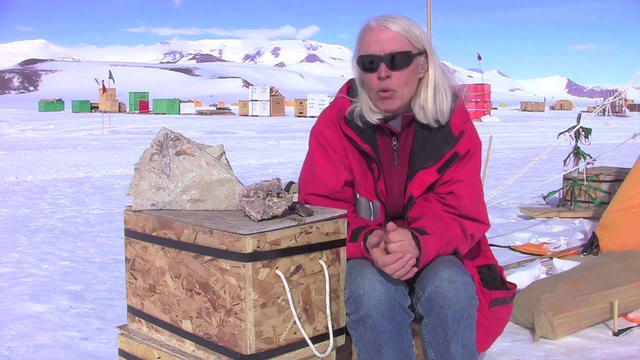 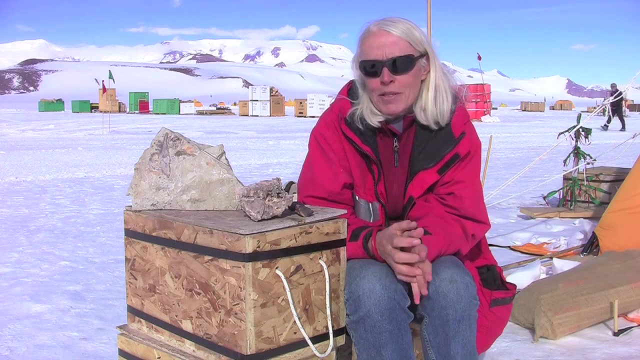 can also, in some cases where the stratigraphy is not known very well, I can sometimes be able to help solving the problem how old it is or how young the plants are. There are many good reasons for studying the plants as well, and one more thing is that if it wasn't for the plants, there wouldn't have been any dinosaurs.